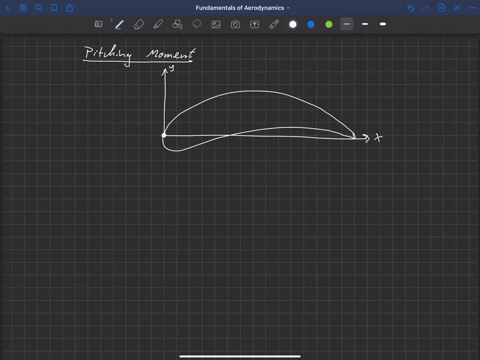 and here's the origin of our coordinate system, right there. Now, remember the force. I can integrate the pressure and the shear If I were to zoom in on a portion of this airfoil. we have pressure- that's always acting normal to the surface, and we have a shear force. 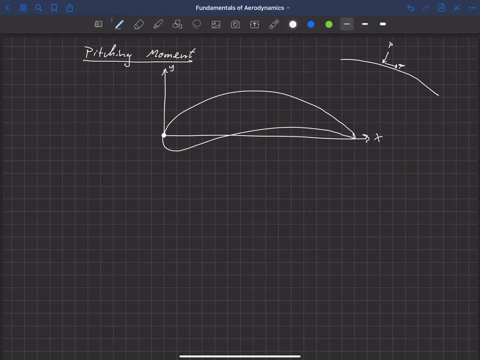 that's a tau there representing shear force that's acting along the surface of the wall. So tau at the wall, that's our shear force at the wall, And so we can walk along this airfoil and integrate all of the pressure forces that are acting normal and all of the shear forces. 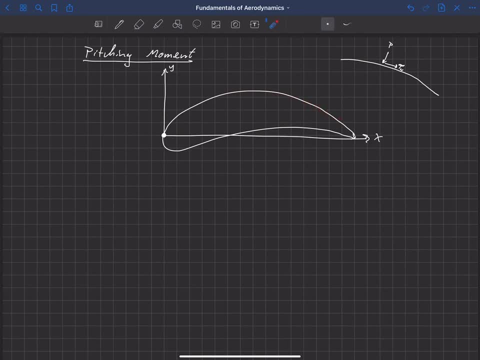 that are acting tangential to the surface, and sum all of that up and we will get a global force coefficient or, excuse me, just a force vector. And I can place that force vector anywhere in this X-Y coordinate system. It turns out that that force is independent. So I'm just going to 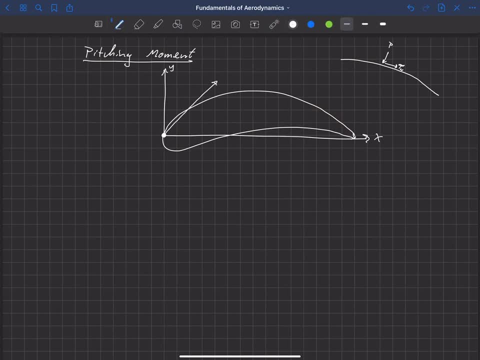 of location. so I'm just going to draw that global force here at the origin. Okay, that's a capital F, That's the force at the origin, And we can divide that into axial and normal components. So I can say there's this much of the force in the axial and normal components. 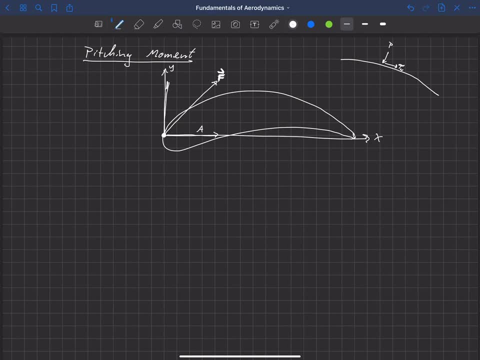 direction and this much of the force in the normal direction and, and of course you know you could connect these, the ends of these vectors there, that that's the magnitude, and the axial direction is an X direction and the magnitude of the normal force in the Y direction. but but the total force is the summation of 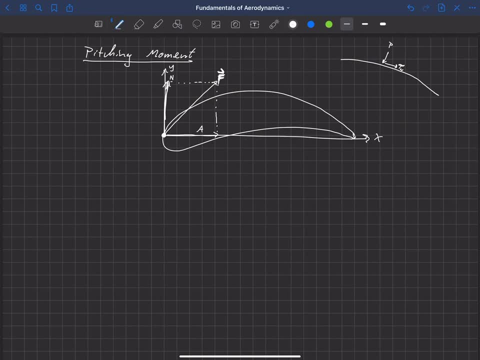 those two, okay, and then. and then we also sometimes like to rotate those forces by alpha. let's say that our incoming velocity is at some angle of attack to the x-axis there, and and so we can actually rotate those forces and talk about the forces that are perpendicular to the, to the freestream velocity, and 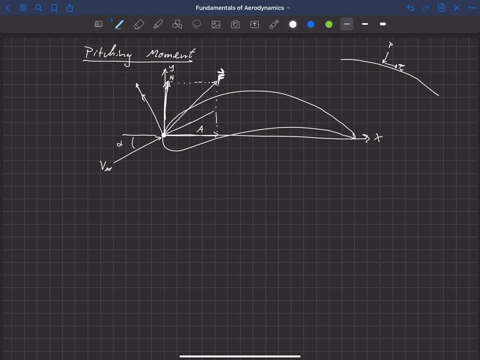 the force that's in the same direction as the, as the freestream velocity. the force that's in the same direction is what we call drag, and the force that's perpendicular to the force that's perpendicular to the force that's perpendicular is what we call lift. okay, and so if we know axial and normal, we 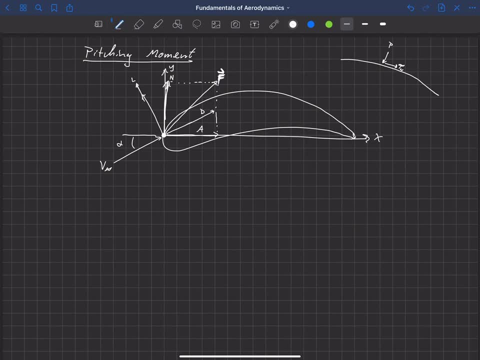 can get the lift and drag. that's just a simple change of variables in using using sine, the cosines of alpha and and same with, if we know, lift and drag, we can get the normal axial by rotating it back through alpha. so in fact let me just write those equations down really quickly. so the lift is equal to the. 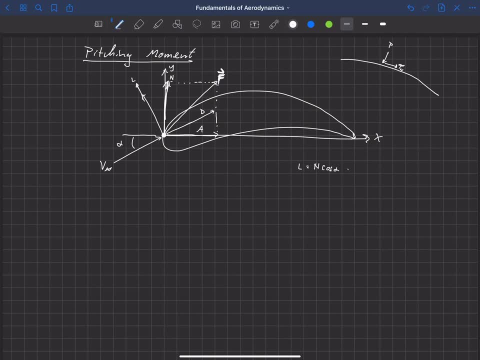 normal force times the cosine of alpha, and then we can get the lift and drag minus the axial force times sine of alpha drag is equal to the axial cosine alpha plus normal sine alpha. and and then if we knew lift and drag and wanted to find normal and axial the, the normal force is: 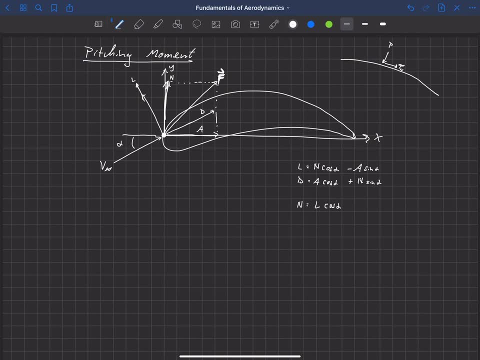 lift times cosine alpha plus drag sine alpha, and axial is drag times cosine alpha times. cosine alpha minus lift sine alpha. Okay, So we can, uh, we can- either get the lift and drag or normal and axial. Okay, So let's now talk about the, the pitching moment. The pitching. 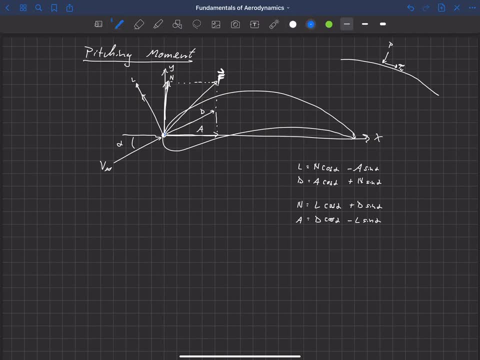 moment is a little bit different. Uh, and I'm going to put this in in blue here. So here's our origin And uh and uh, when we, when we walked around this airfoil and summed up all of, 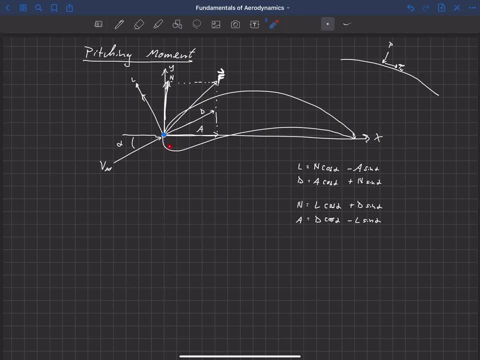 the forces. it didn't matter about what point uh, we were summing those because, uh, those just had a direction. So so, each of these, uh, these forces, as we integrated along, had some, some force in the axial direction and some force in the normal direction, And we basically summed those. 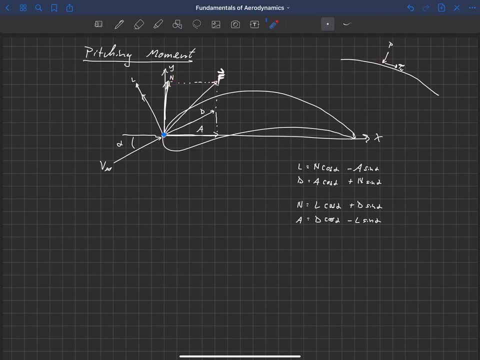 up in order to get a normal and axial or the, the total force. But, uh, when we talk about a moment, we we are summing those forces about some location on the airfoil. So, uh, a lot of times we'll choose the origin in a, in a computational world, It's, it's, it's nice to. 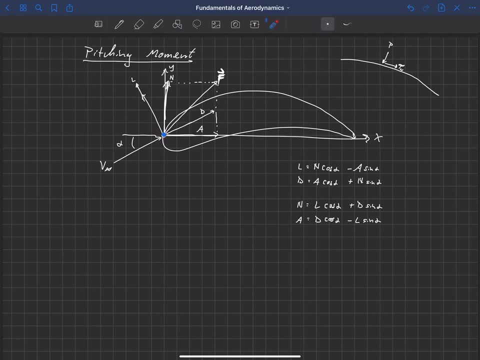 choose the origin. Uh, if you're in a wind tunnel, this is equivalent to somehow pinning the um, pinning the airfoil somewhere, or or setting some sensor, Um, and I'll just, I'll just draw a pin. 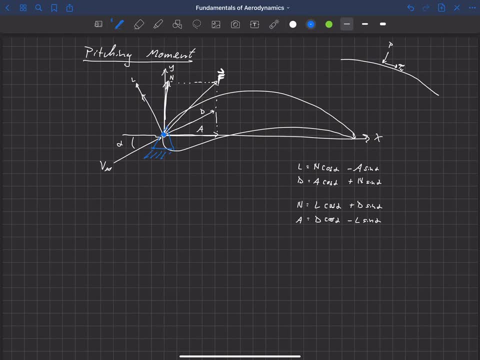 For example: uh, if we were to pin this airfoil here at at the uh leading edge, then, um, and and put some sensor at that location, We could figure out how much moment the aerodynamics were creating about that point. 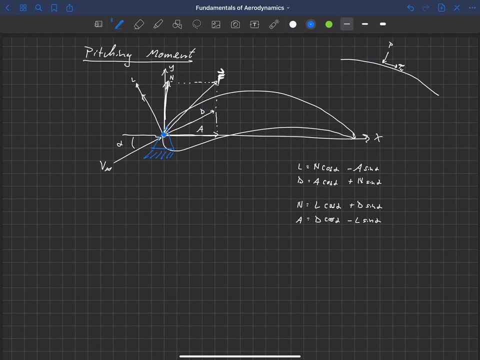 You know what was the strength of the torque? basically, um, on that airfoil, about that point, Uh, okay, So let's take off our, uh, our pinpoint there, but, um, anyway, we need to choose a location. And so, if I zoom in on this uh surface over here what we're doing basically. 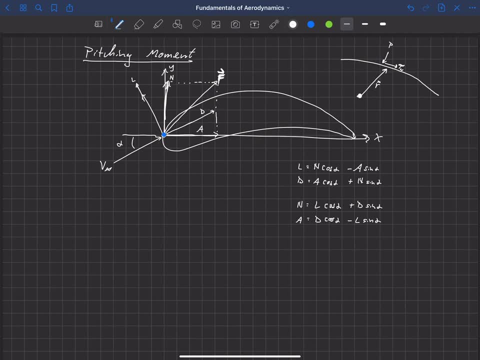 is, we're walking around the airfoil and we're saying I've got some distance R from the point of interest which usually is is the origin here. Um, but uh, I've got some, some point of interest and I know the the distance from that point. 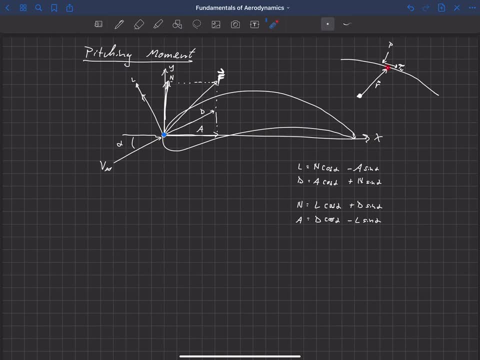 to uh to this point on the surface, that I need to uh compute the moment about this point, And it turns out that that, at the surface, that uh, there's a total force. I'll use a little F vector: total, total force, uh. 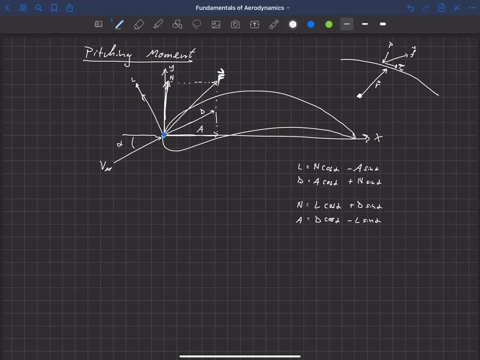 to pressure and shear And, uh, if I take the cross product of that force with this radius, then I can get the moment, uh, that that is um creating about this point. Okay, So, as we integrate, so so we're going to integrate now along this whole surface. 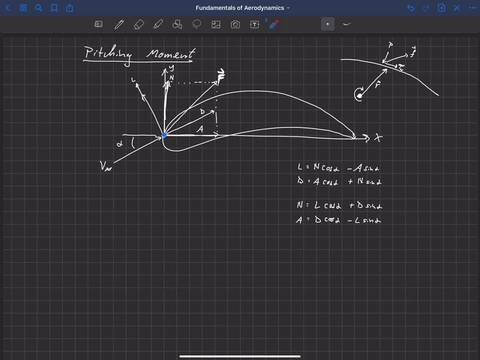 we're going to walk along the whole airfoil and um, integrate the, the shear and the pressure forces about some location. So let's choose the leading edge and um, and we'll get some uh, pitching moment. So I'll just draw. 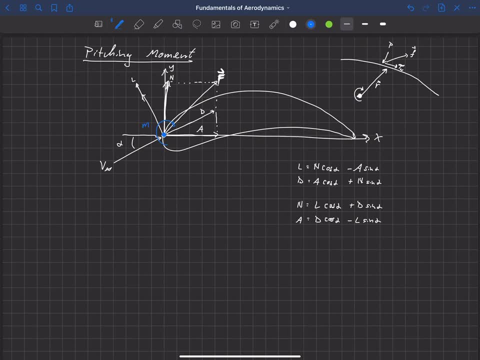 uh, that moment. there We we use a little M and um, uh, and now you know we've measured that about some point. but sometimes it's useful to know what the pitching moment is. What if we had summed that about some other location? So I'm just going to put some 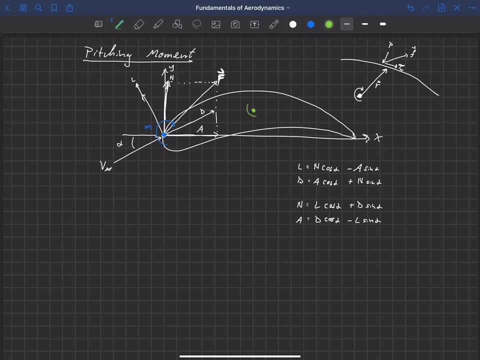 other location here, uh, and say that I'd like to know what the pitching moment is at that location. And, by the way, we're going to subscript the, this first moment, with a Z, uh or an O, meaning that's the pitching moment about the origin. And now I'd like to know the 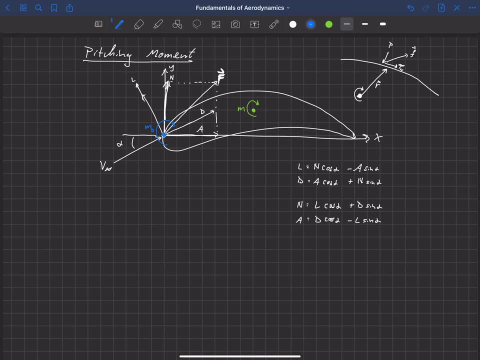 pitching moment at another location. Well, it turns out that I don't need to reintegrate my- uh, my forces and moments around this. I can actually just take the known pitching moment at this location, as well as the the normal and axial forces, or this total force. 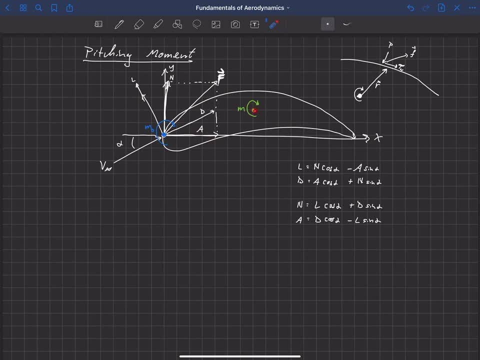 and uh and compute what the pitching moment would be if I were to uh, compute it about that point And uh, it turns out actually even move the forces over there If I were to to measure lift from that location or 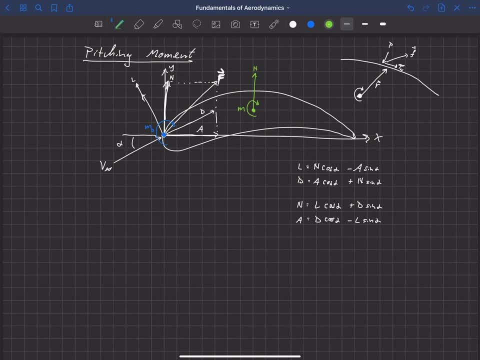 or normal and axial forces. uh, they would have been exactly the same as uh, as they were computed about the origin because, uh, those forces are independent of where I'm computing them about. It's only the moment that depends on this location, Okay, So, uh, so let's write the. 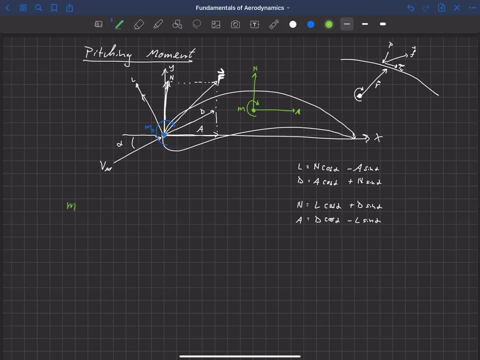 the equation for the- the moment at any location is equal to the moment about the origin. So let's write the: the equation for the- the moment at any location is equal to the moment about the origin. Uh, and then I? this is just a statics problem where, uh, you know the moment, I can just move. 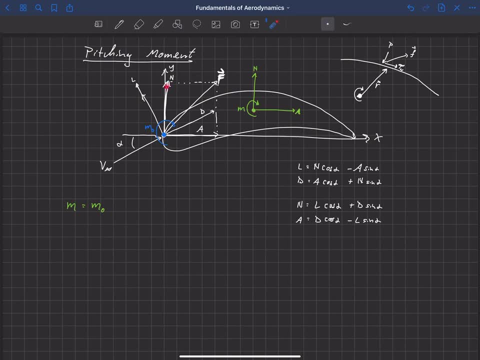 over to that point. Uh, and then I'm going to take the normal force times the change in X, and and uh, a normal force will create a positive pitching moment about that location with positive X. So I would say, uh, it's the moment at the origin, plus uh, X times the normal force. 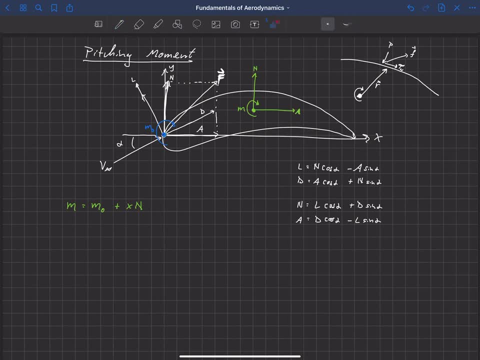 And uh, and then, as I move from from this location to here, if I have some positive axial force that actually creates a negative pitching moment, uh, when I get to this location, And so it's going to be the axial force times the the Y distance there, Uh, and that's going to create. 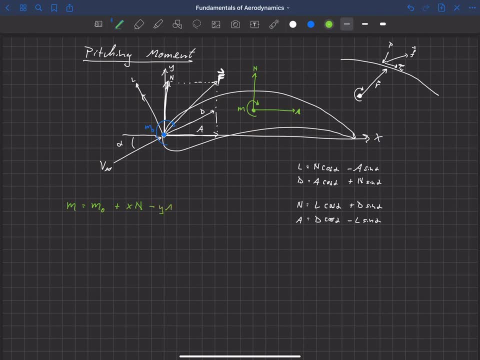 a negative pitching moment, So it'd be minus Y times axial force. So this equation now tells me the pitching moment at any location on the airfoil. Uh, if I know. if I know the pitching moment at the origin, uh, and I also know the normal and axial forces, or if I know. 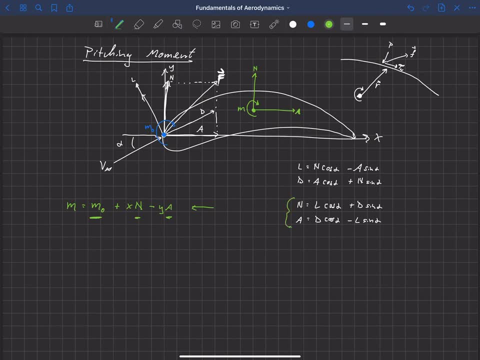 uh, lift and drag. I can get the normal and axial from this equation here. In either case, uh, I can get normal and axial And uh, and if I know the pitching moment then I can plug this in to find the pitching moment at any arbitrary uh, X and Y location. 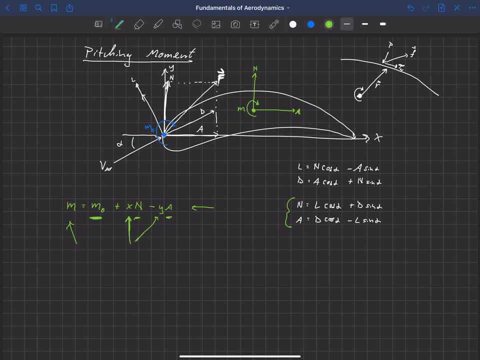 on the airfoil. Okay, So I can just plug in any X, Y location right there and get the pitching moment, And then I can plug this in to find the pitching moment at any arbitrary location. So, uh, in airfoil analysis a lot of times we end up working with uh results that 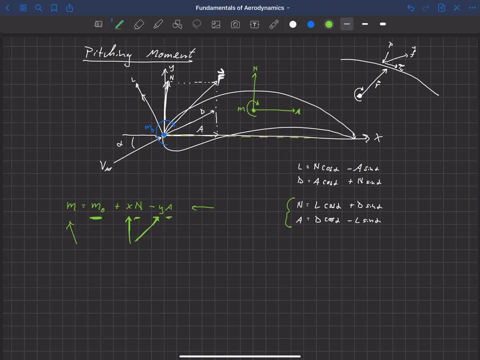 are just right on the chord line here. Uh, but, uh, but that's just a, a that's uh. it just turns out that, um, that a lot of important things happen very near the chord line, And so a lot of. 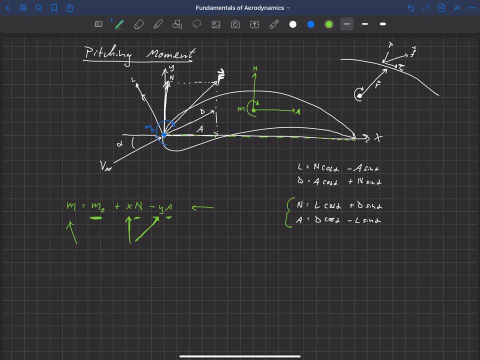 times we just assume that we're working on the chord line, but in general, this is the equation here: uh, that we're interested in, uh for pitching moment, And it depends on both your X and Y location. So part of the reason that 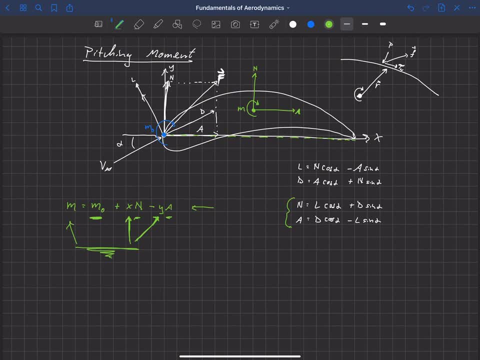 we, we sometimes just look at the chord line- is um. let's just look at the components of this equation here really quickly: Um. so if you look at the X offset, um, X can go, uh, you know, from from the origin all the way back to the chord, Usually the Y offset of this region that. 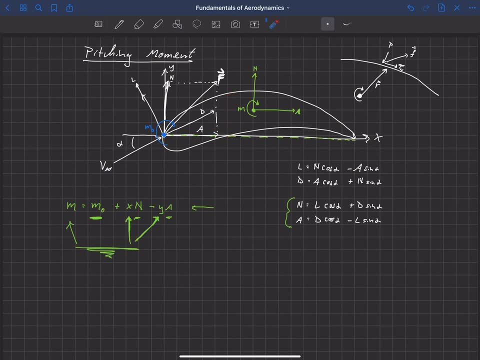 we're interested in is pretty small compared to X, because these airfoils are rather thin. they're usually on the order of eight to 12% thick, uh, percent of the chord, Okay, And so, um, if you look at X compared to Y, X is usually much larger than Y And uh, and, and also our normal 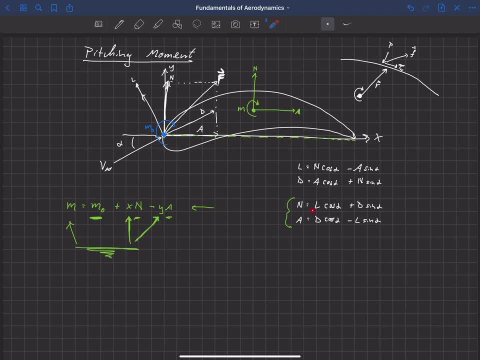 force is, uh, is closely related to lift. So so it's, uh, it's an offset of you know, lift times. the cosine of alpha also has some drag sine alpha, but but, uh, in general our normal force is much. 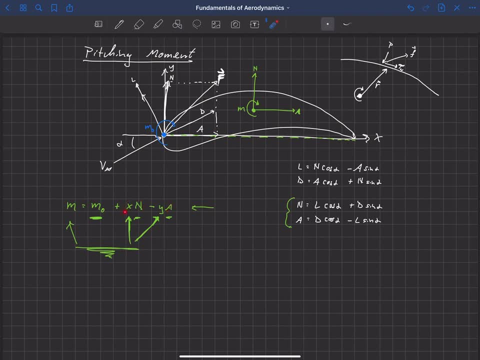 smaller than our axial force. And so you've got two large values here, X and N, and you've got two small values here that are multiplied together that even makes something smaller and something larger here, And so, um, a lot of times we'll just look at the pitching moment along the chord line.